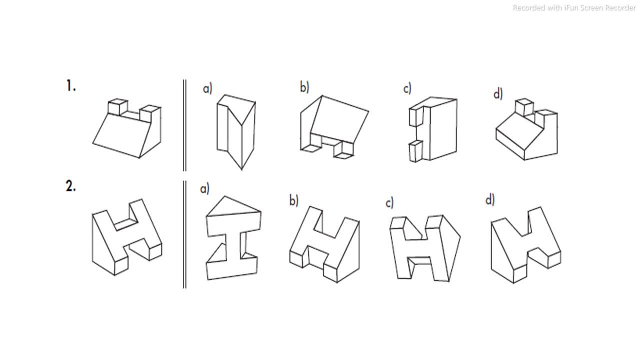 come across the figures related to the rotation of images. it is more of your analysis capability, how you perceive pictures and how good you are in analyzing and the rotations of images. if you are good in analyzing the figures, it's very good for you to solve these questions easily, but if you are not able to rotate these, 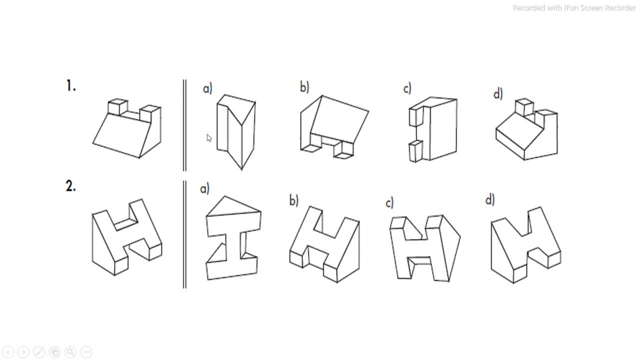 images in your mind, picturize these rotation images in your mind. so you don't have to worry about it. you can still figure out how to solve these questions. the method we use here is the elimination method. so to to figure out which will be the rotation images of this, we will try to eliminate which are: 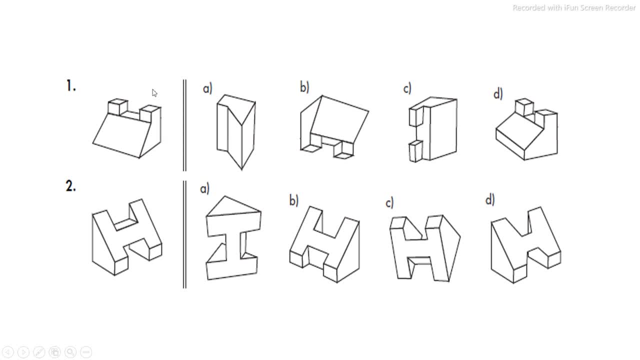 not, and then we'll land up with our answer. for example, if we see in this picture, we will try to figure out which one is the most prominent in this figure, like if I see this picture. so first one of what I see is this keyword, like structure standing. 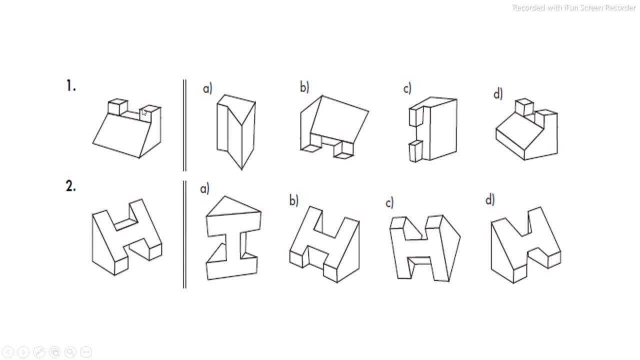 on the clip on this structure, right. so we'll see which kind of figure in this is having this. so with based on that, we'll try to eliminate the figures which are not having this kind of a structure. if we go with the figure A, you can see. 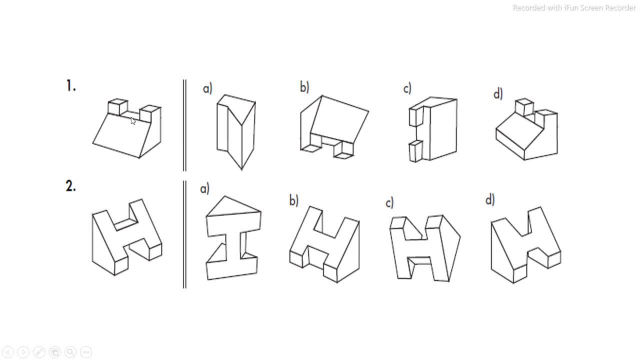 that in this, between these two things, there is a gap. but if you see, from this, it is a straight going forward from this to this, which means there is no gap. so this cannot be our answer, so this cannot be our answer. so we'll cross it, then we'll move on to next. so we'll 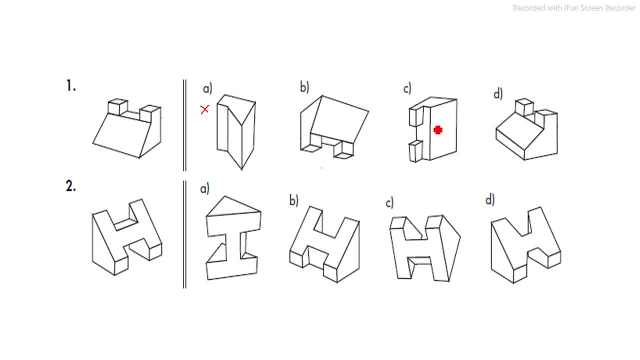 see, this figure is there, so this can be our answer. now, moving on to this, so here you see that this box is coming in whole width of this right. this is whole width. but here, if you see, this is coming only up to half of this right, this half a. 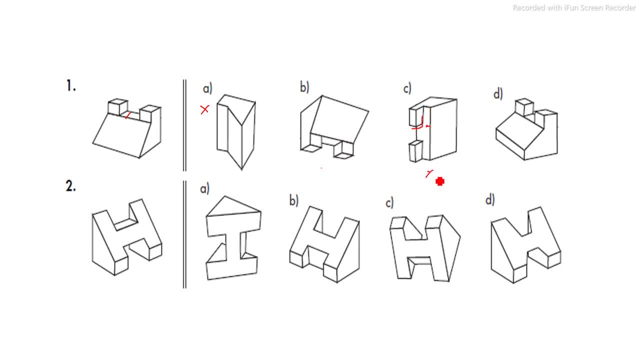 space is empty, so this cannot be our answer. this is wrong. now this is also coming full to full, so this can be your answer. now we'll have to compare between these two. now we'll see this figure. if you see this structure, this is coming straight to the downward, because if you see in this figure, you are seeing in 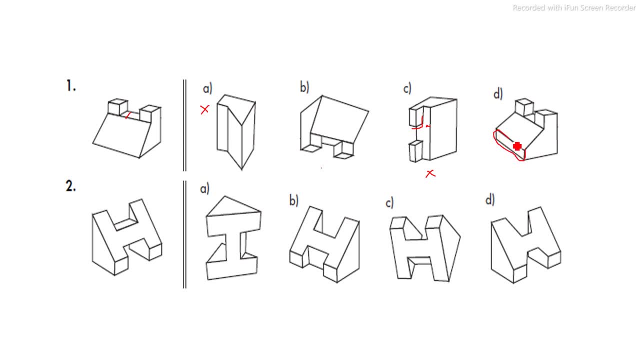 this structure as well, an extra layer of this thing, but so which is not in the main figure. so this cannot be our answer. this is eliminated so. hence, three figures are eliminated, so automatically, the fourth one is our answer. so with this logic, we are going to find out the. 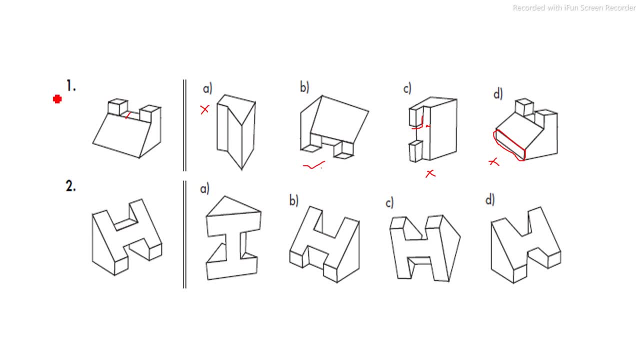 answer for the rest of the things. so the thing is, you might be seeing that while analyzing these questions you are. I am taking very long time. this is because I am explaining the things into you, but if you do these things in your mind you will be quite fast, and maximum it will take 40 to 45 seconds to solve this question. 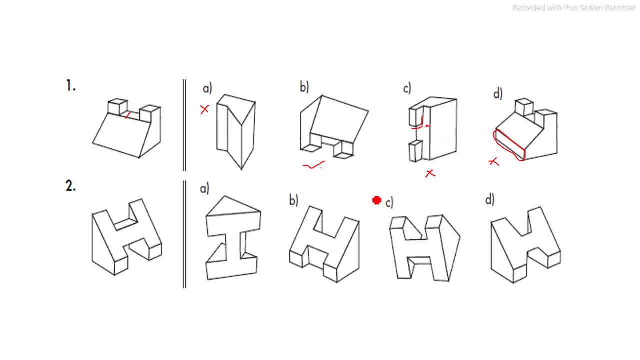 so let's move on to the next question. to practice more and understand better. since question number two, here see, we will first see. there we can see the prominent one is H structure. right here we are seeing this H structure, so we'll see which are having H structure. so this: 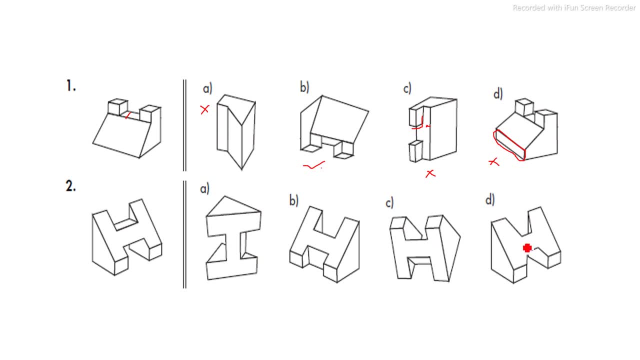 is having H structure, this is having, this is having, but this is having a different kind of H, right? so this is inclined H. so that is not our answer. so this is eliminated because yeah, if here you see this is inclined, but here if you see it is straight line, right. so this cannot be. 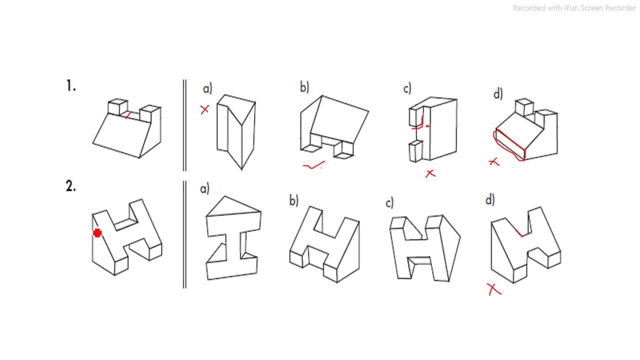 our answer. now we'll move on to our next thing, that is, this structure we can see right. so our shape is like: here: this is, then this, then this and then this. this is the same. so here we see only triangle we are seeing. so this is wrong now in these both figures. 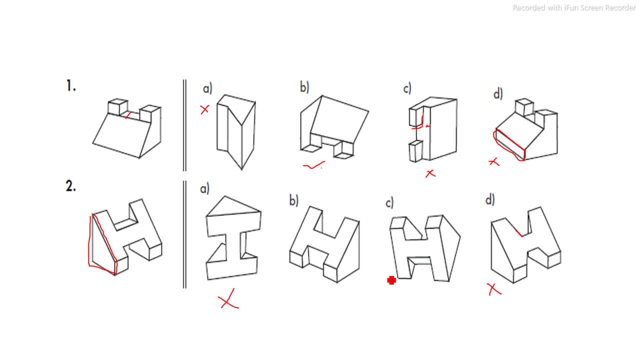 the same structure there. so these two can be our answer now to further eliminate. we'll see this structure. you see, this triangle is there, this forming of triangle is there right now. you'll see where it is. so in this you are seeing, with this extra structure, this four. 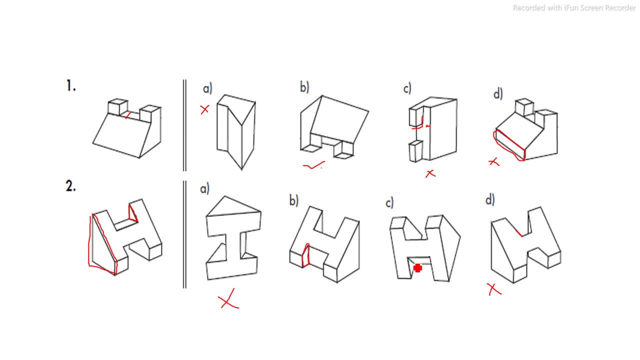 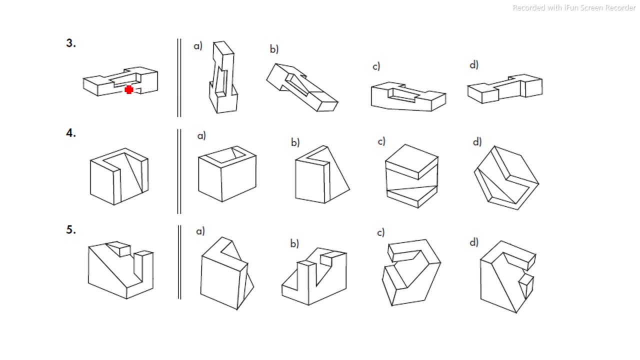 side of structure is there, but here this is triangle, triangular one which is identical to this one. so this is eliminated. so this is our answer, moving on to next question, so this is third answer. what we can see here is, as we see, if we see, we can see the eye structure right, a sleeping eye. 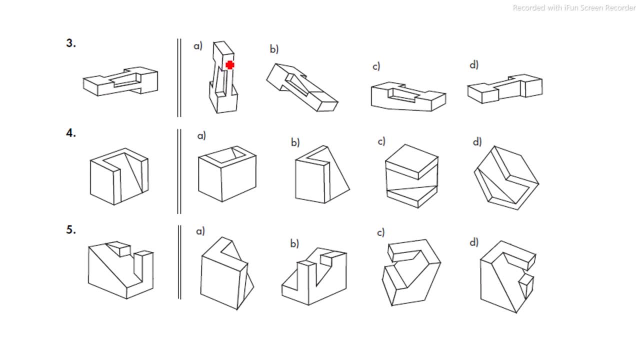 so we'll try to eliminate based on I. first, here we can see: I structure. this can be our answer. here we can see: this is a a bit of T structure, not I. so this is eliminated. here we can see: I- this can be our answer. and here we see I. this can be our answer. now, moving on to what we see here is: 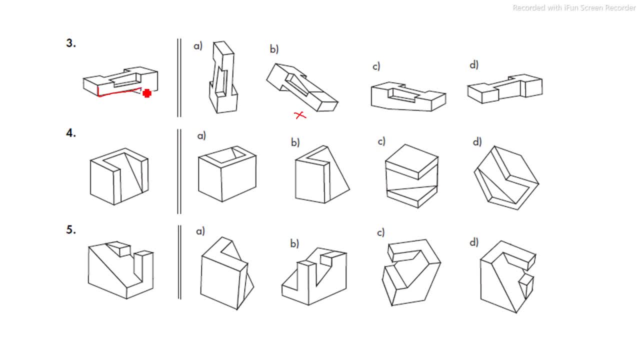 so let's see, focus on this structure, right, this is there, this kind of structure. so this is there in this one also. okay, then, if you go by this, this is already eliminated. now, if you see here in this figure, if you see this place right in under this, this is empty space right there, right, but here, if you see, 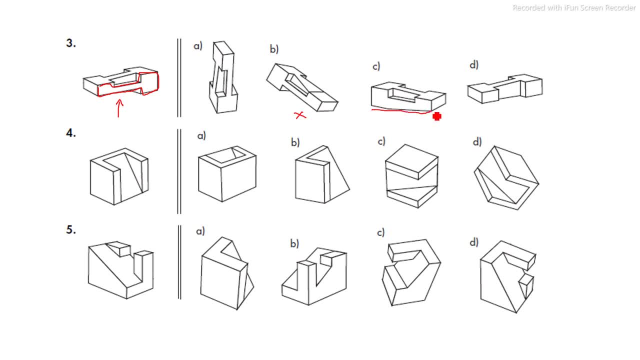 under this slot, a full, full-fledged structure is there. so this is also eliminated. no empty space here. if you see, there is above empty spaces and there below it is empty space. so this is eliminated. and this is also eliminated because here you see this i structure. 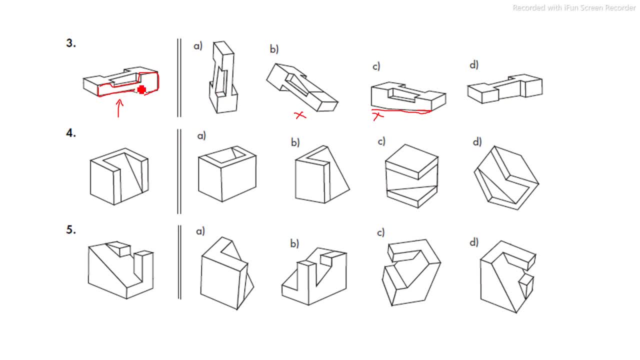 and this slot like structure is there. but here you cannot see any slot. right from top to bottom it is empty. but here, if you see there is a empty thing like a structure thing, so if you go by this structure formation, so this structure formation is not there, so this is eliminated. but if you see this one, so this structure. 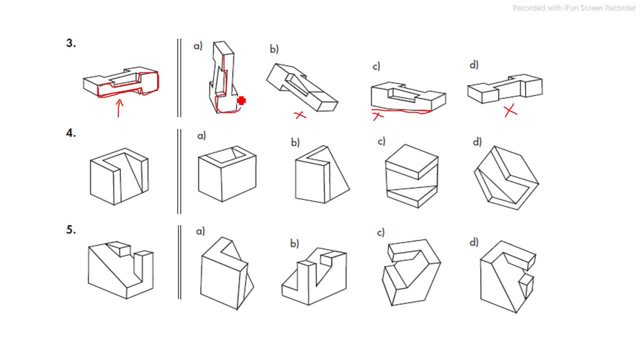 formation is there, right? so this is our answer. moving on to fourth, so in fourth, if see, we'll see what. uh, this is like you like a structure, right? this is you like structure, so we'll see which is having you like a structure. here you, we are seeing you like a structure, but 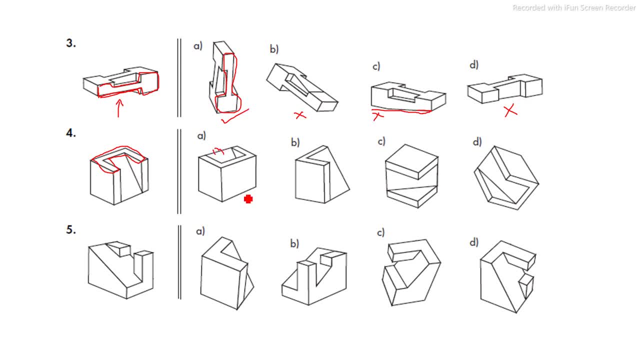 it is a closed one. here we are saying it is open, so it is eliminated. here it is directly eliminated because this side is not at all there. so this is eliminated, because here you see, there is one side and there is second side, but this second side is missing. so this cannot be our answer. 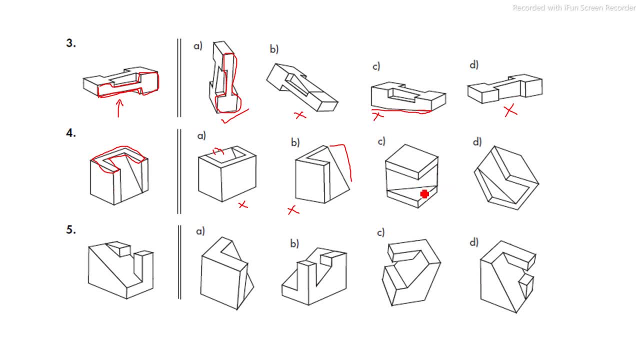 now moving on to third. so here we can see, two sides are there, but here, if you see this, you like a structure, it is missing double line right here it is only single line. so this cannot be our answer. so this is our answer. moving on to question number five. 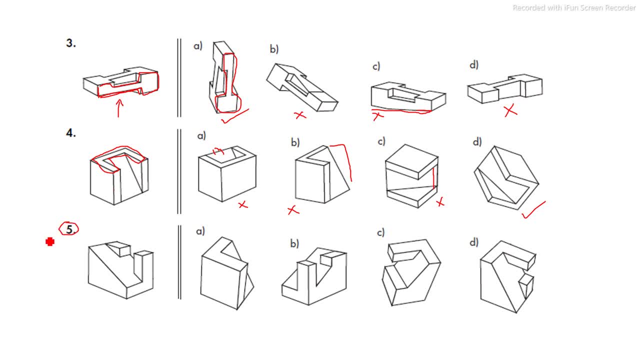 so remember i have said you have to pay special attention to it. so it is a. so you need to have a different kind of approach, not completely different, but have a different level. so we'll figure it out while solving it. so in the first thing, we see this: there are 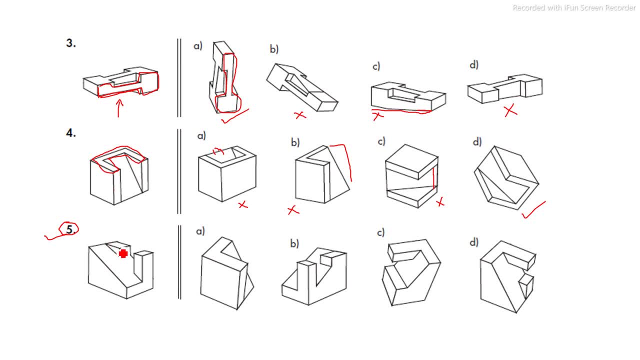 one pillar like structure and this is another pillar perpendicular to it. right? so here in this figure, no pillar structure is there. this kind of pillar is not at all present in this, so this is eliminated. now this can be the one we are seeing, this one, this one. 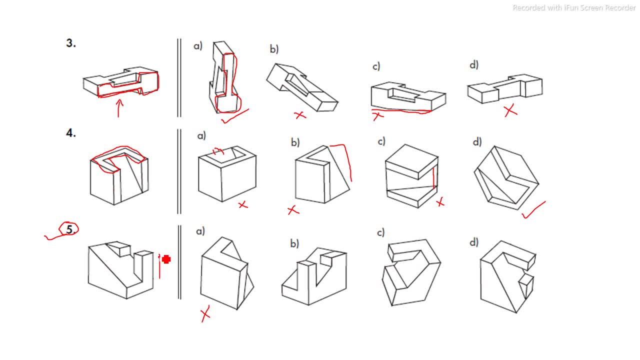 and now, coming to this, there is one pillar we see, but the second clear is pillar is missing. we cannot see this kind of perpendicular pillar against this. so this is missing. this cannot be our answer now. moving on to this b and d, so these probably can be our answer, because we are seeing this pillar like structure. both are there right. 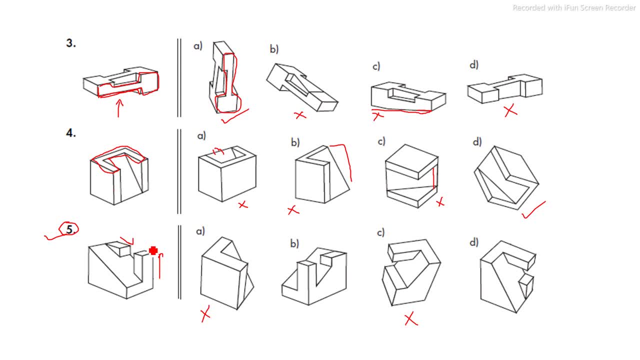 now here. what is the catch is, if you try to go by the logic which we are going in the above up to fourth question, we are seeing, like, if you see this, there is a triangular structure right here, right, this triangular structure, and if you go here, there is no triangular structure you can find, but here. 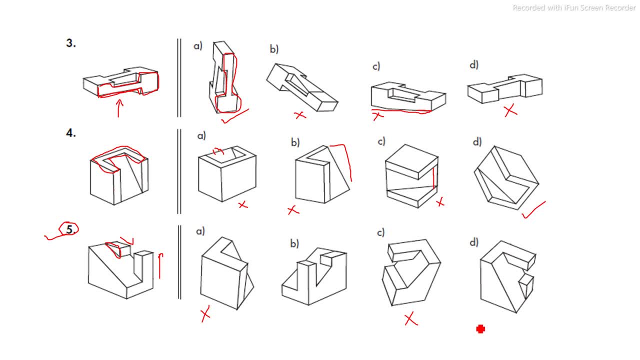 you can find this triangular structure. so with that logic, this would be your answer. but this is not our answer. why? because if you see similar kind of things, you have to think of mirror structure as well, because in most of the questions the question setter gives sometimes mirror images. 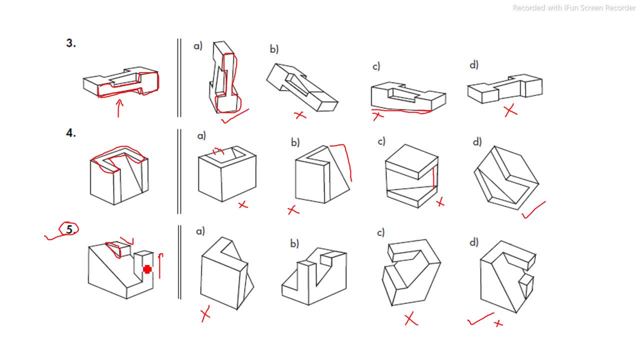 of this. so if you see, here we have to visualize a little bit, use our analytical skills to understand these questions. now, if you see this kind of thing, the pillar, if you see the pillar here and the pillar here right, so this pillar is on the left side. if you try to rotate this figure like this, 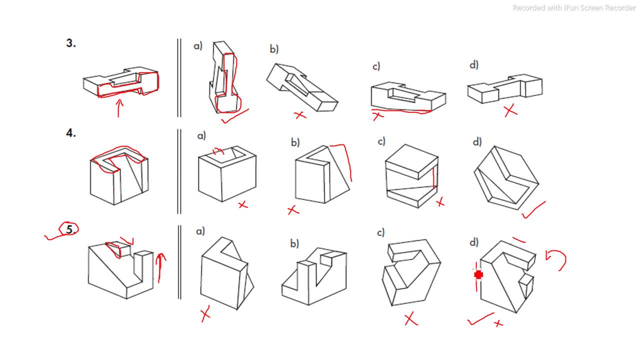 and make this figure stand on this, like this figure. now, this figure is, this portion is standing like this. make it like this. so this figure and this pillar, like structure, will come here. so what i am trying to say is that when you rotate this image to your left and make this structure stand on this base, you will see. 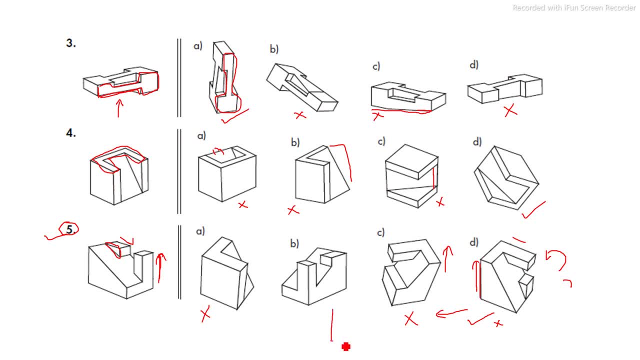 that this pillar is coming to this side. this pillar will come to this side. this will be the some kind of structure and this will come here, some sort of things like this. so this can be a. this will be a figure when you rotate this. but if you see our main figure, this pillar is to our right side. 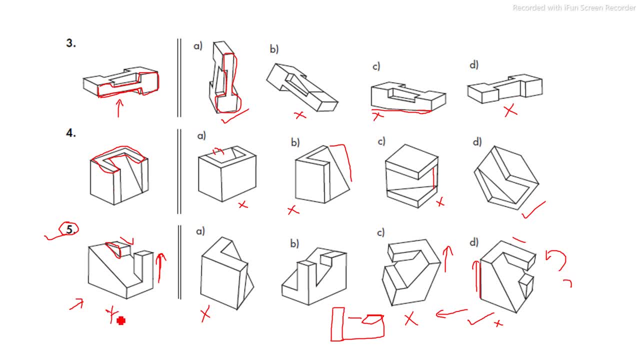 like, if you are standing here, if you are standing here and if you see, the pillar is our, this long pillar is our right side, right. but if you see, while rotating this, what we find out, that this long pillar is coming to our left side, right. so this cannot. 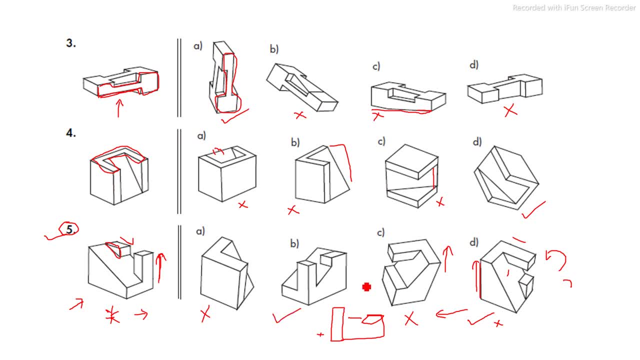 your answer, so this will be our answer. so you have to be careful while solving these kind of questions. I hope you are able to get this thing if you. if not, then please go back and see it again so that you can understand the things, because a year we will have the mirror images moving on to next. so we are with 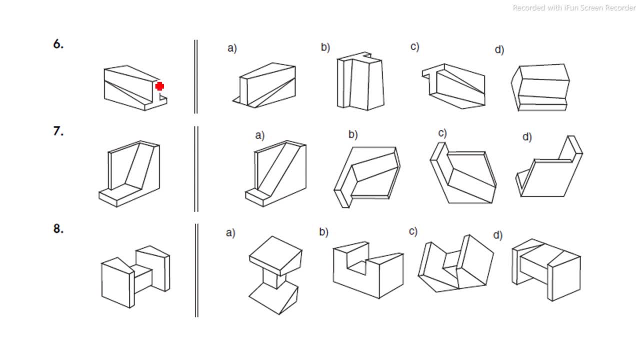 the most permanent thing we can see here is a reverse T upside down T. so here you will try to eliminate based on this. so here the T formation is not there because this piece is missing. so this cannot be our answer. now you are, there is T, so this can be our answer. there is T. this can be our answer here. 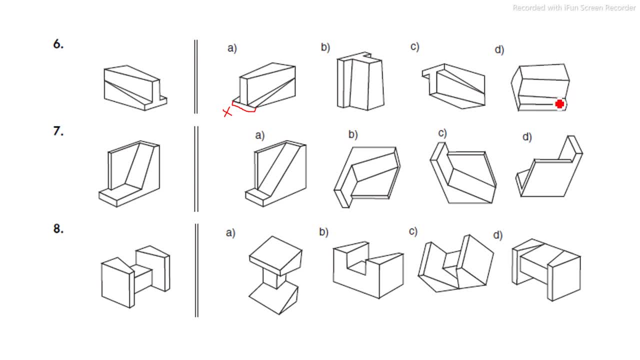 no T is at all and even if you see the side view, so if you can see the side view, there is one. these two, this path is a broad here and this gets pointed here. but if you see here, this path is broad here and this is a little. 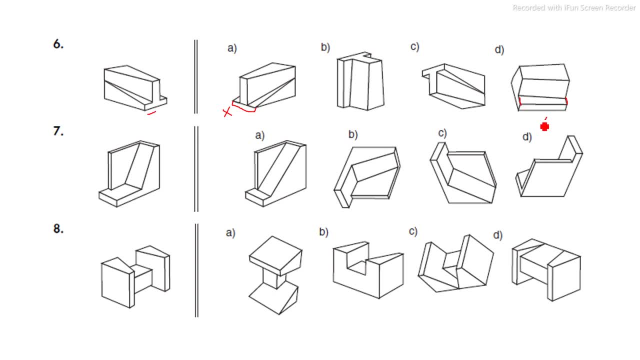 narrower, but still broad. so this cannot be our answer. you know here the same logic: this path is getting convulsed to a pointed fall, but here, if you see, this is not at all pointed. so this cannot your answer. now, ultimately, this will our answer, so you? 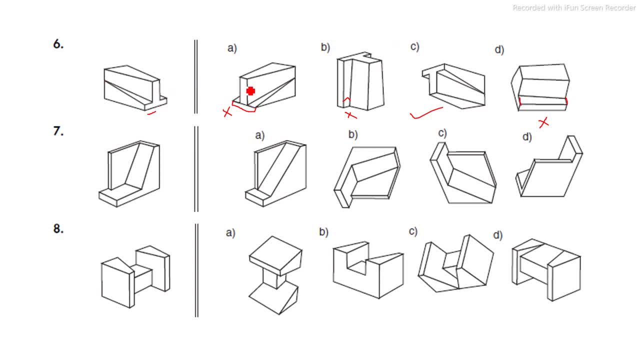 see that you don't actually have to rotate the things and figure it out in your mind how the pictures are rotated. you just have to eliminate which cannot not be your answer and you will land up on the correct answer. now moving on to seventh. so here, also remember, this question is also some sort of different approach. we'll see what the different 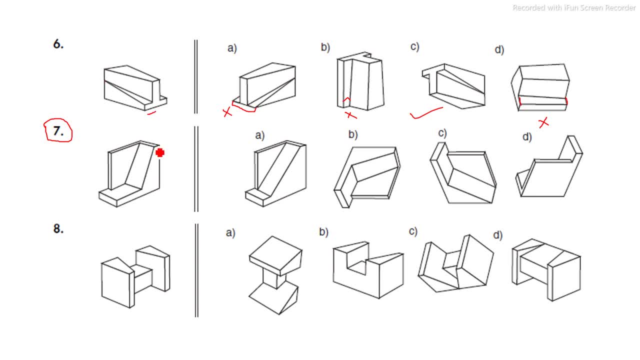 approach is here. so first of all, we'll go with the traditional way. like we are seeing a sloping, there is a sloping and this l the sloping. l like structure, so this is automatic. this is very prominently eliminated because this is very less kind of space. here we see, this is a more spacious. 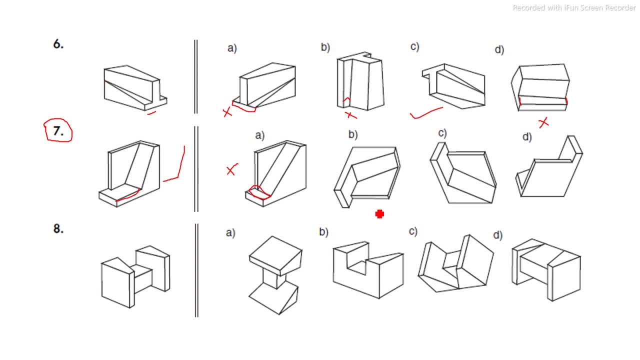 as compared to this. this cannot be your answer. now coming to these three figures. so here if you see, like if you see in this figure, you cannot see anything right, because this is we are seeing from this side. so when we see from this side, so this portion of the figure will be hide out, so we 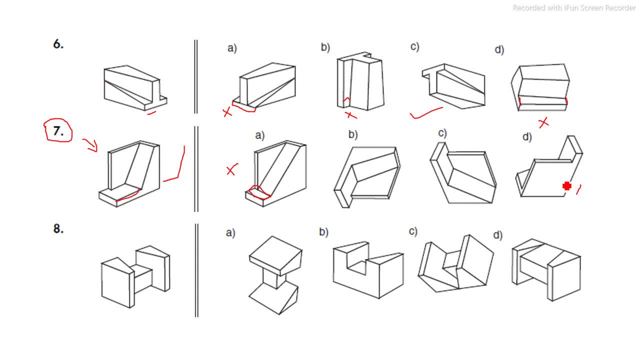 cannot see this person. so this is from that view. so we cannot directly eliminate it because we are not able to see through it, so we'll have to wait for the elimination method. so now, if you see here, these two are quite a look alike and these are looking like it can be our answer, right? 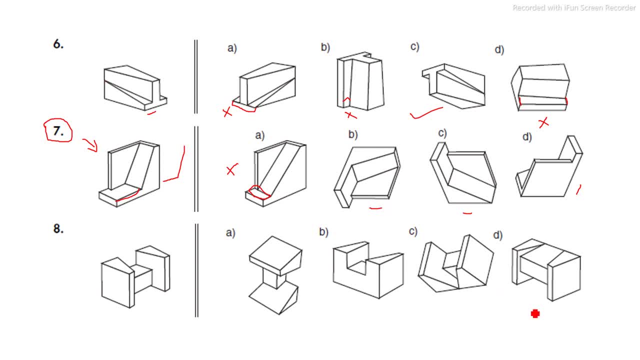 so we'll try to figure it out. so first let's go with b. so if you see here, uh, the structure is very similar. we are having this: two lines are there? two lines are there. so this is two lines. are there up to this? here also two lines. here also two lines. so all are perfect. every structure is aligning. 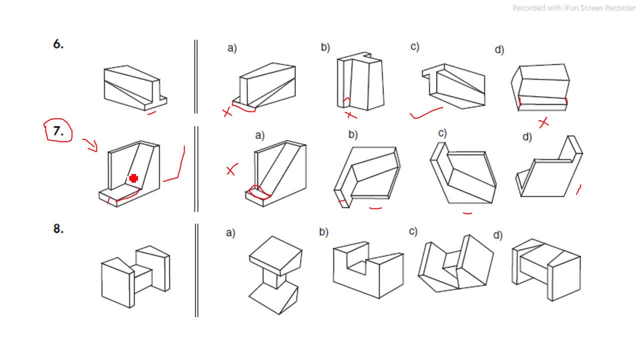 okay, then we have to. what we can see here is that this can be, and we have to check whether this is a mirror image or not. so how we'll see. so imagine if you are standing, if you are sleeping on this slope. right, imagine you are lying on this slope. 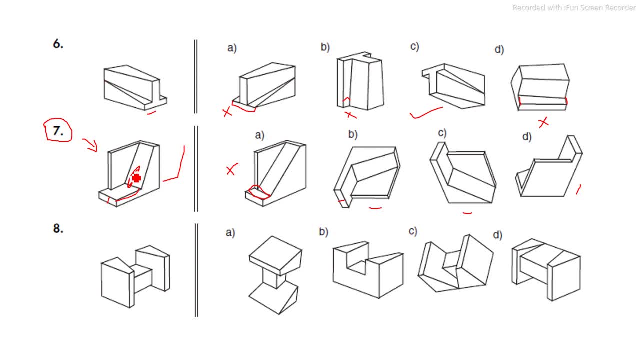 so what, you see, that this wall like structure will be on our right hand side. so if we, if we imagine ourselves standing this on this slope, so this wall like structure will be on our right side. and when we do a similar kind like if we stand on this slope, 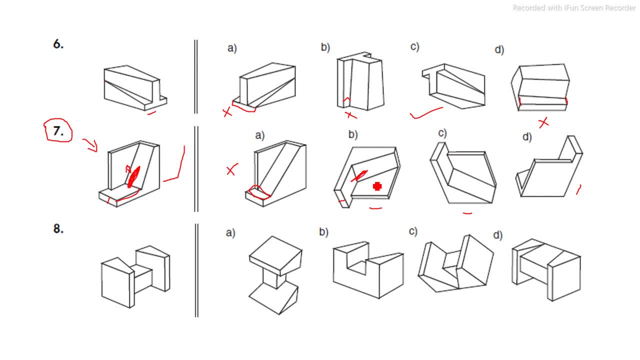 and if we see where is this wall like structure, so this will be coming to our left side, right. so in this we are coming, this structure. if you stand this on this uh platform, you will see that this wall like structure is coming to your left side, so hence it cannot be. 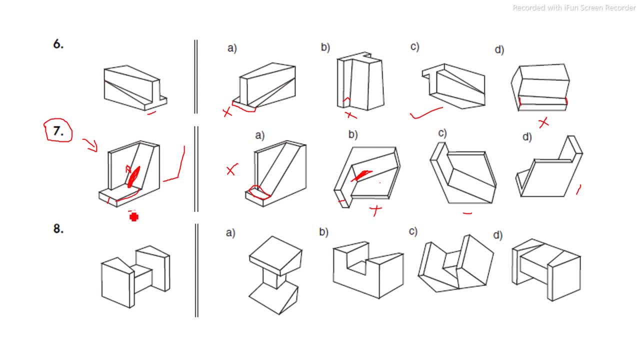 our answer because, uh, the left of, because the right of this is coming to left, which means it is a mirror image. so mirror image cannot be your answer. so this is eliminated. so if you see that this figure was quite identical, so if you were in hurry, or you will go by previous logic of 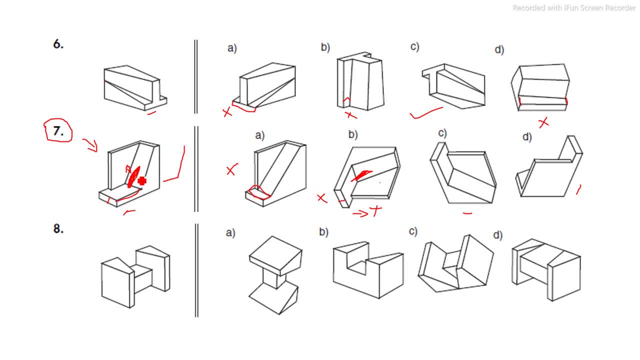 understanding that all the figures are there. figures are there in aligned, aligned form. this structure is matching with this structure. this double lines are matching with this double line structure. so you can mark up wrong answer. so here you have to analyze that also now if you come to this. so if you see here there is double line on 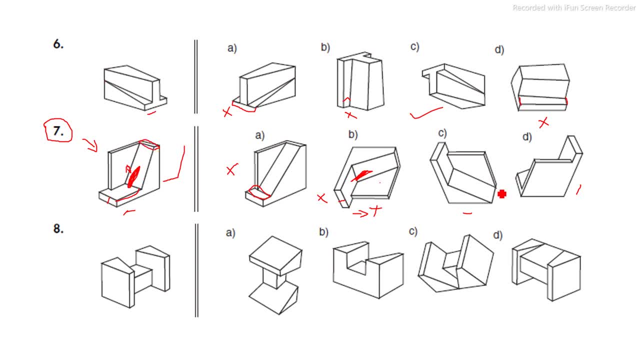 the slope right, but here only single line is visible right, if you see this wall like a structure, and the double line continues till here also. so this cannot be our answer. so ultimately our answer is this: so you can see here what is special about is this: that if you directly say: 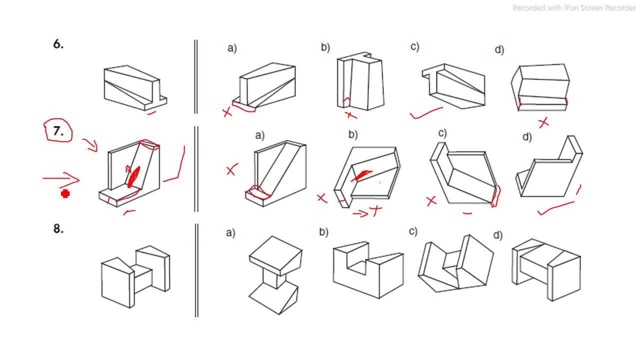 and directly see things without knowing anything. if you go by this simple logic, you will directly mark this as not your answer, because here you are seeing a slope- right, this is a slope, but here, if you see a straight line, is being shown right. so it will definitely mark this as. 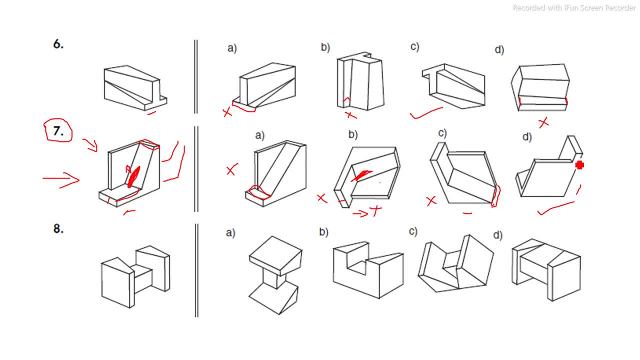 wrong, but this cannot be, because this is upside down. if you correctly analyze, the slope is from here, only the slope is here and this structure goes like this. so you don't have to do in the analyze that much. but if you want to verify, you can verify with this logic. so any questions? 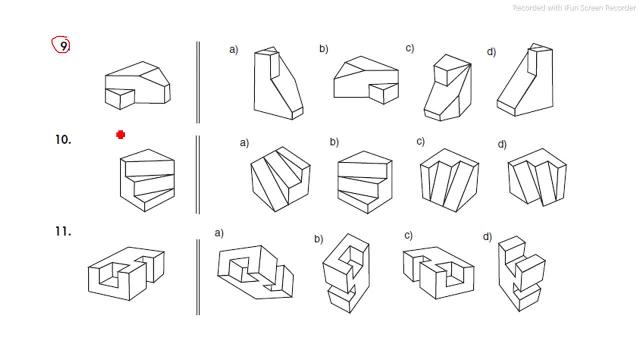 so this is also one of the special cases you need to understand here, and this is the most special case because the most this this is having the most surprising answer. so we'll go by elimination method first and we'll see what happens. so, if you can see, there is a 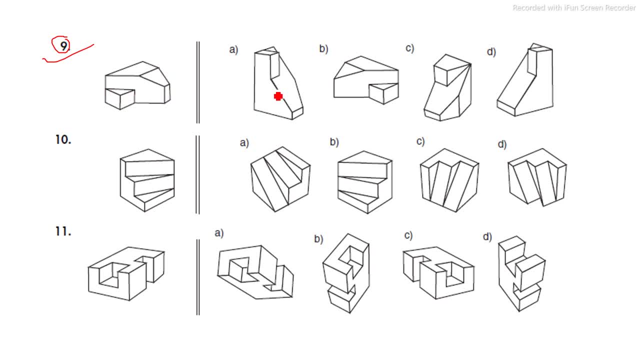 the, this triangle, like structure you cannot find here, because this is completely different structure what you are seeing here and you cannot imagine that this kind of structure is also possible with this. but we cannot mark it as wrong. why? because we are not able to see any any sort of structure. 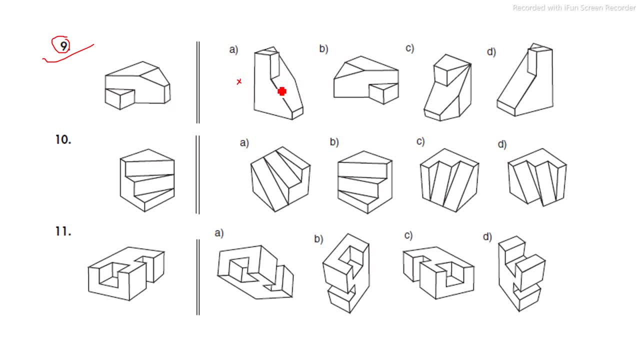 things like: so we cannot mark. maybe it is showing some different kinds of view which we are not able to figure it out. so this can, this can be our answer, because we have not find out anything which can prove that this is wrong. so here, if you see in this figure, so here it is clearly wrong. why? because if you see, 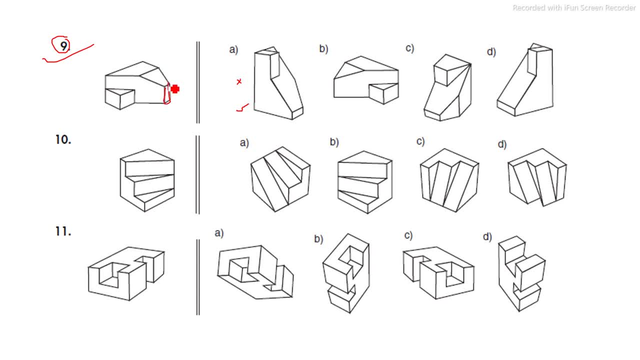 after this slope here. this is a double line, double line structure, right, but here you see, for only a single line is there, double line is missing. so this is a clear case of no answer or it is an odd one. so this cannot be our answer now, moving on to this. so, if you can see, there is a triangle like a structure here, but 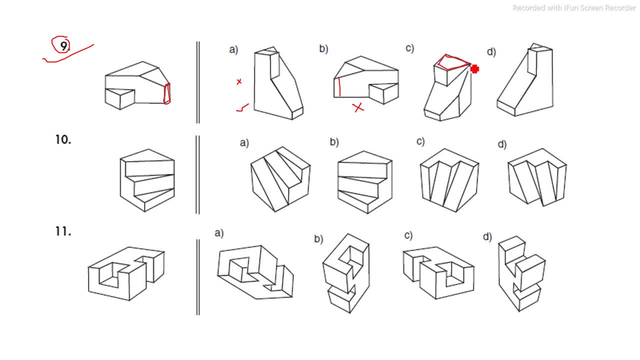 here, if you see some sort of square like structure, is there right, not a square. the four sides are there, so this is prominently wrong because here, if you are seeing, this structure is there and this is completely different from what we are having in the main figure. so that is why this is wrong. 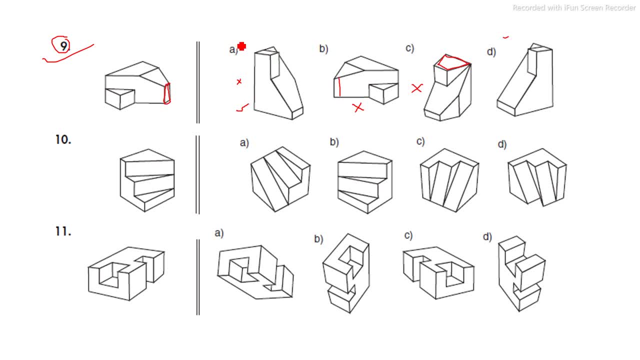 now here with these two figures, d and a. if you see a and d, we cannot see any kind of similar structures with this, but we have but and this kind of figures were looking like. this can be your answer, but these are eliminated. so now how would i figure it out which one is right? 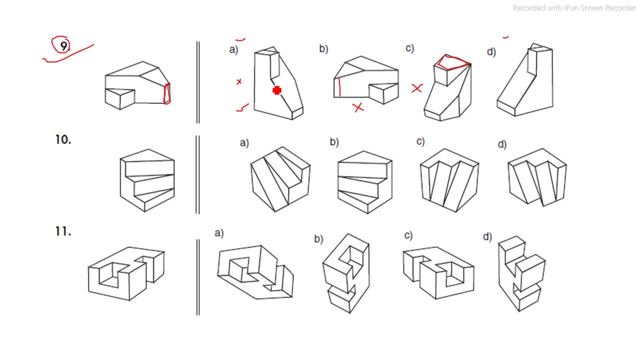 so here we have to understand a little bit of logical things, like if you try to analyze this figure and this figure, so what? you can see that this slope like structure right here, if you see a slope like structure, and here, if you see this is a straight line structure. now, if you go by this one, 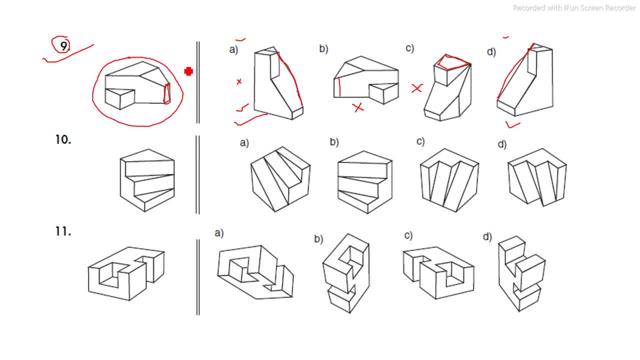 if you analyze this figure at any point of view, you will see there will be a slope. if you see from this side, so you will see this slope. right, if you view from this side, you will see this slope again. if you see from this side, you will see this slope. 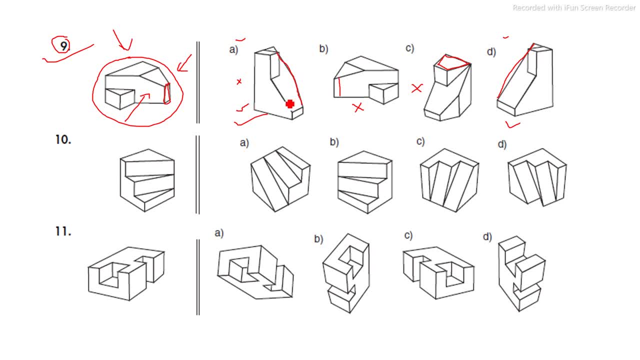 right. but when you go, but when we see here this is a straight line structure, right, this is a straight line structure. so this is eliminated, because in no case we are having a straight line. in every case we will having, we will be seeing a some somewhat of slope like structure, as you can see in this figure. this is one. 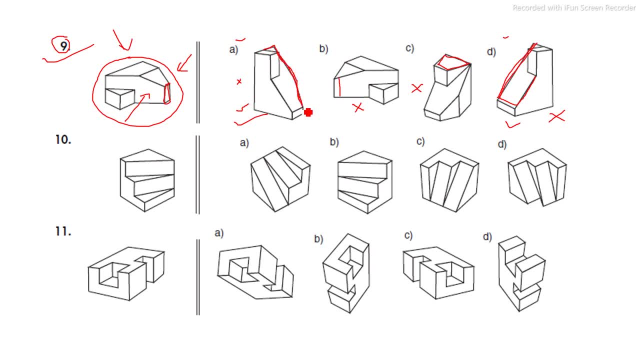 this is a bit slope and then this is a bit slow, right, so this is our answer. i know that you may be thinking that this kind of logic is not being applied because, like, uh, you you'll be thinking that how this can be your answer. but this is: if you analyze, this is a different kind of view. 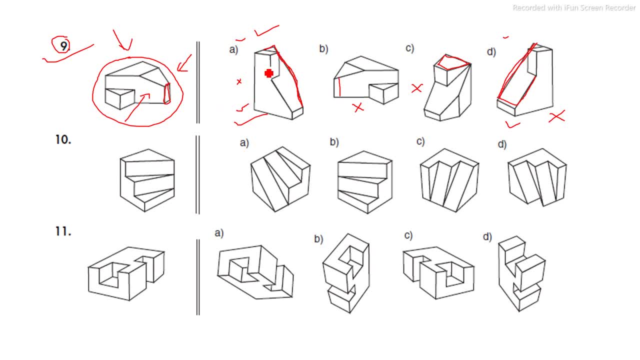 so if you, if you will try to figure it out which kind of view? it will be very complex and you will- this understanding of this will require a huge, uh, i would say very analytical skills in your mind to understand these things and rotate the figure to make this figure it out. but in the competitive 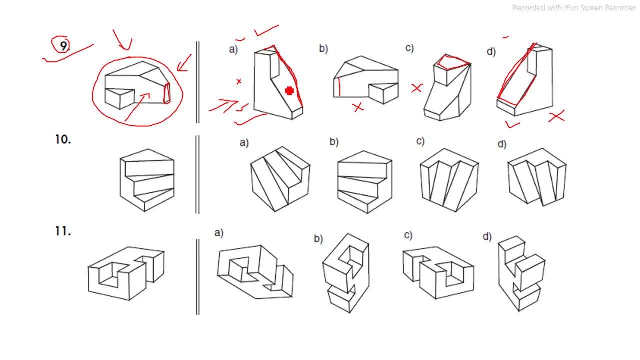 examination. we don't have that much time and we are not doing a thesis that we need to understand things. we just have to mark the correct answer right. so these three are wrong, based on the things which are prominent that this cannot be. this cannot be our answer, because we ultimately have: 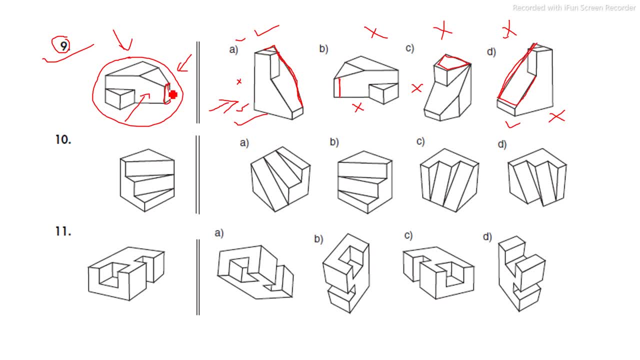 seen that this: there is a double line and here we are seeing only single line. so this cannot be our answer. here we see four lines. here we see three triangle line, triangular structure. so this cannot be our answer. here we see a complete straight line from top to bottom, which cannot. 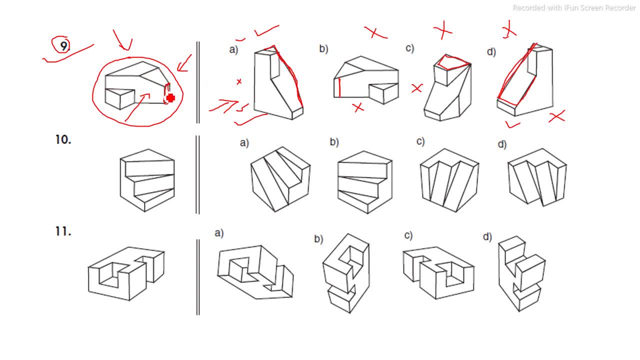 be possible because there is a slope. from any side you will see a slope like a structure. so this is our answer. so that is why we are looking at this problem, why this is a special case. moving on to next question, so here also we'll try to figure it out by the elimination method. 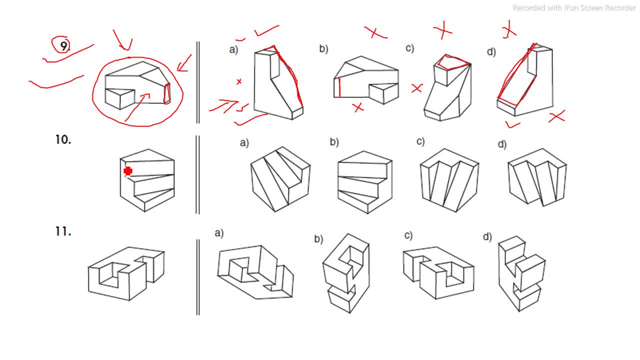 we'll just go by this staircase structure, right, you'll see this stair like structure. so here this is eliminated because this staircase is not complicated. completed one steps is remaining here, so this is eliminated here. a step like structure is there here. step like structure is there here, also there. now we have three figures. 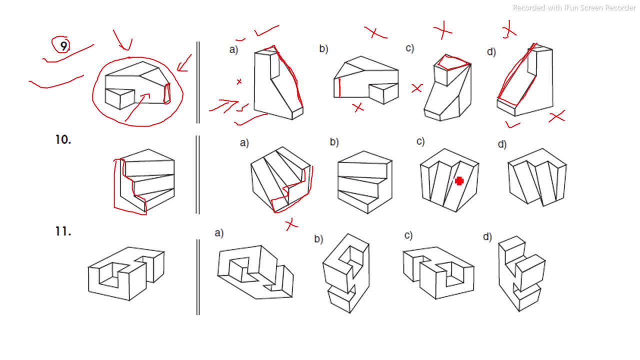 now we'll go with now. if you see them, they are very identical to each other. but if you see this figure, this, this triangle is completely. if you see, this triangle is here, there this is bulging out and here this is lagging behind. but if you see, in this, 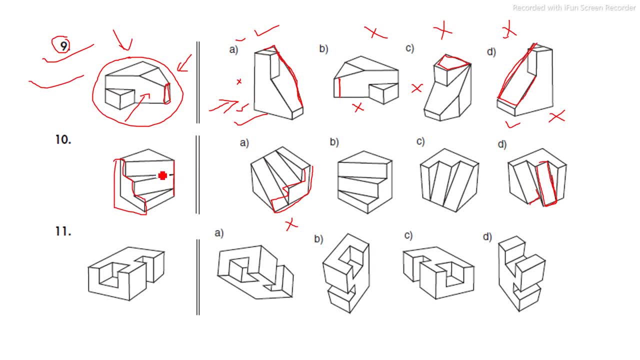 triangle are aligned to each other in one line, like this triangle is up to this and this triangle is aligned, but here this triangle is here, then this triangle is lagging behind. so this cannot be your answer. this is eliminated now. these two possible answers are there. now you are seeing that. 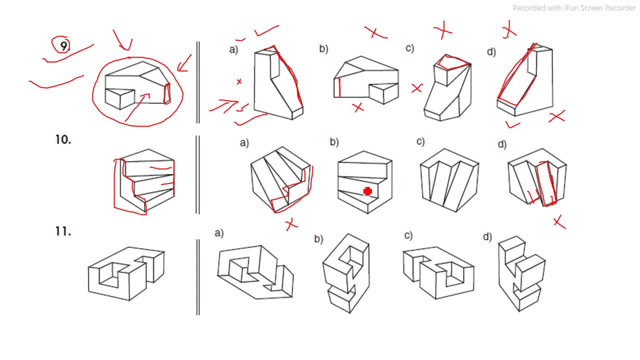 there is very identical in nature. so we'll try to rule out the method whether there is any mirror structure or not. so how will try to find out mirror structure? so here we don't have to think very analytical that we'll try to rotate in images in our mind. all you have to do is that what you 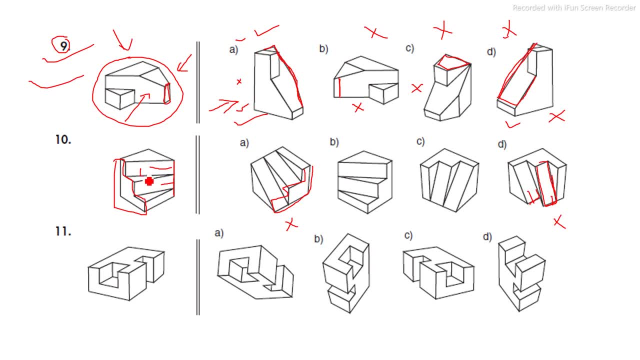 can do. imagine that in this main figure, you are sitting on this, on this stair right. you are sitting on this stair and your face is on this, on this structure. right. you are seeing this structure and sitting on this stair. so now you what you see that this, this figure like and this: 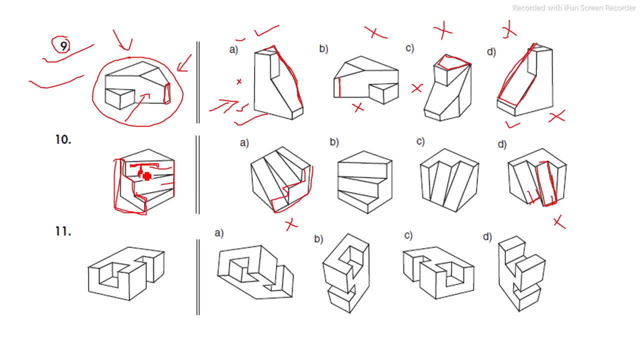 wall like structure, will come to your right hand side, right, if you are sitting on this stair and watching this wall. so you, this stair like structure will come to your left hand side, right. similar thing will try to do it here if we are sitting on this staircase watching this wall. 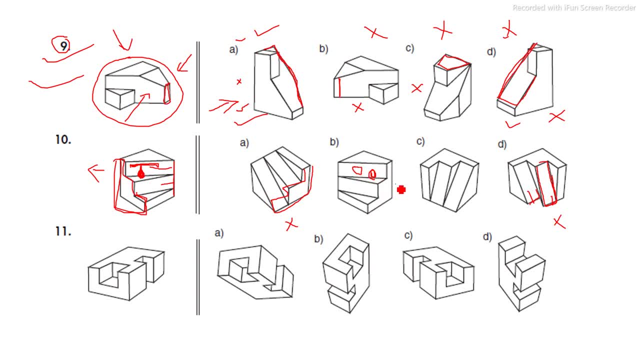 you. so this stair, like a structure, will come to our right hand side, right, so definitely here we are having in left hand side, here right hand side, so this is a mirror figure. so this is eliminated and this is our right answer, or otherwise, if you think, if your mind clicks very early, you can see, if you 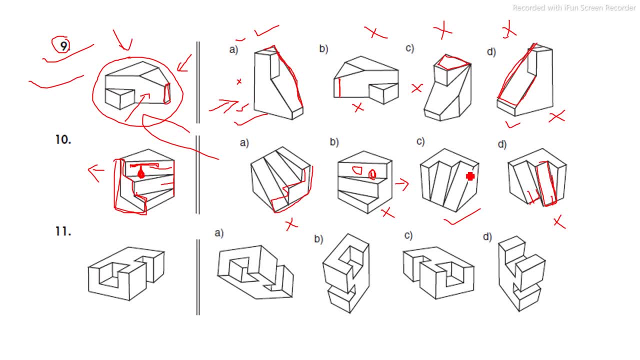 are good at rotation also. so you can see that if you rotate this figure, this like this one here, and have a feeling that if you rotate this in this way, there will sudden load of this one, so even lend up and this figure. moving on to the expression- and here it's a- we can clearly 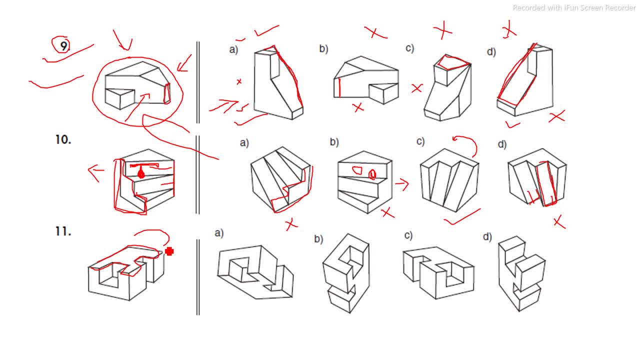 visualize. that's a widget, so if you try to rotate, it is like this. so if you write to rotate this structure, we will try and end up things like a y like structure, something like this: right, so what you have to distinguish here is that where is this term if you rotate this? so this: 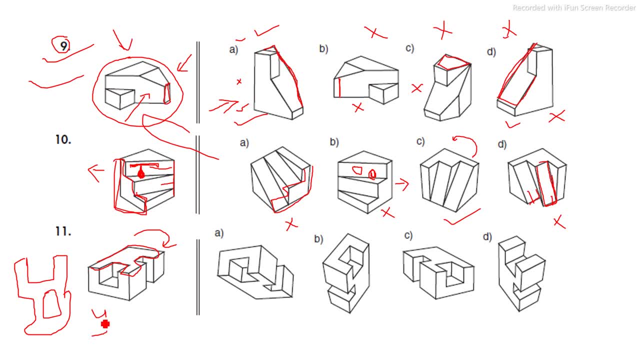 term will be like this: this is the structure. so we'll have to find out where this structure is for me. so here, if you see this y, so this turn is there here, like the. in this, the figure is like this: this is u and the figure this turn is on the right side, so this is eliminated. here, if you see, 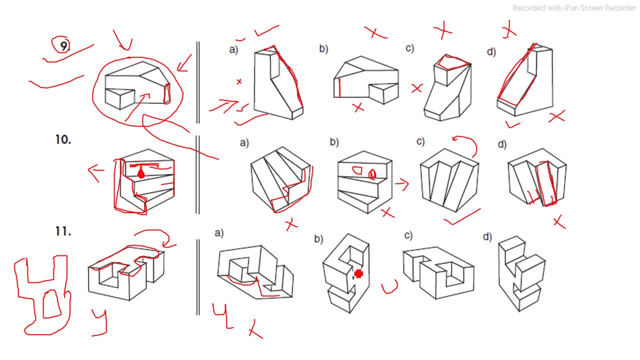 this is there. this is there here. here you can see u is there, you go down and this is there, so this is matching with this, so this can be our answer. now we'll see other figures as well. so if you rotate this image, this like this one, so you will see this. if you rotate this image, so you'll see this, y like. 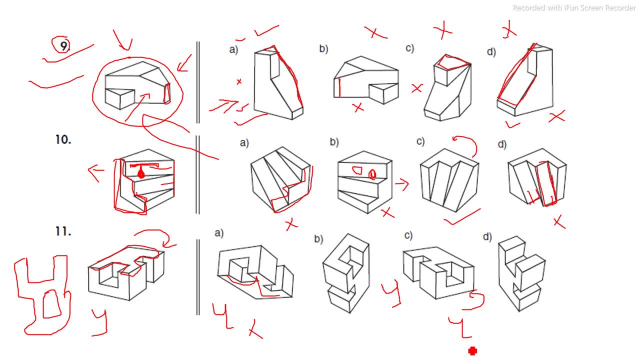 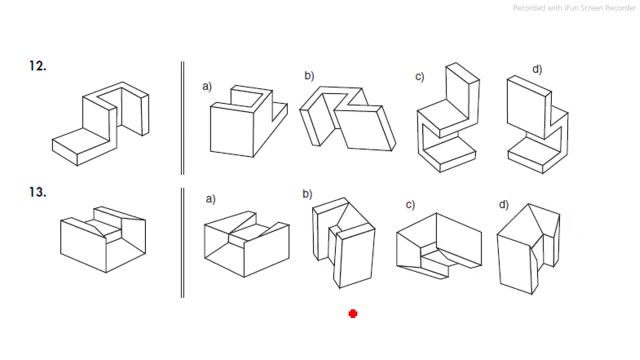 structure and this figure will be here. the tail will be in the right side, so this is eliminated. here also, it is prominently saying this is like this. so this is eliminated. so this is our answer. moving on to our next question, so here we see that we can see this. u like a structure, right? so we'll try to find out. 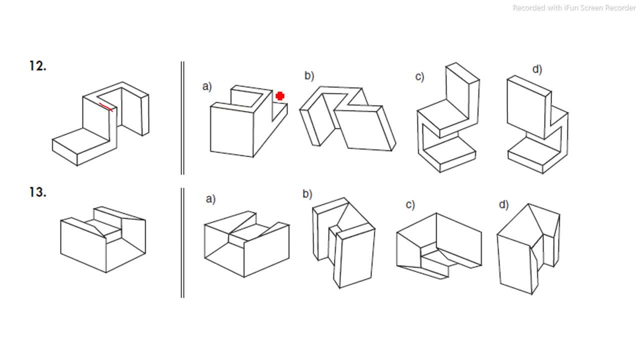 u like structure is everywhere there or not, so it is there in this. if you see here: so this is u like a structure, but this is a continuous one. you go from there to there, here to here and here. but if you see in the main figure there is a stoppage, right, this stoppage is there. so here it. 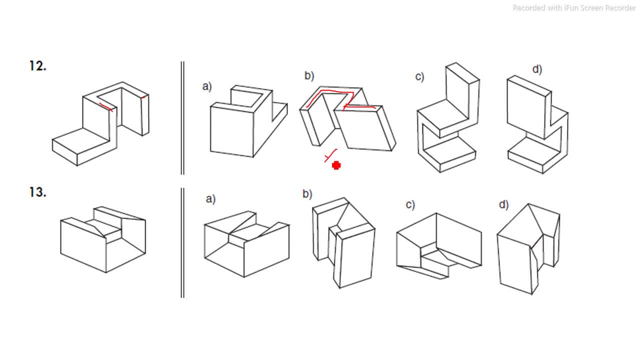 should have been a stoppage, so this will be eliminated. here also, the same thing goes. you are seeing a continuous figure. you can go from here to here, to here, so this is the also continuous, so this is eliminated. now we are left with this and this, so we'll have these both look identical. 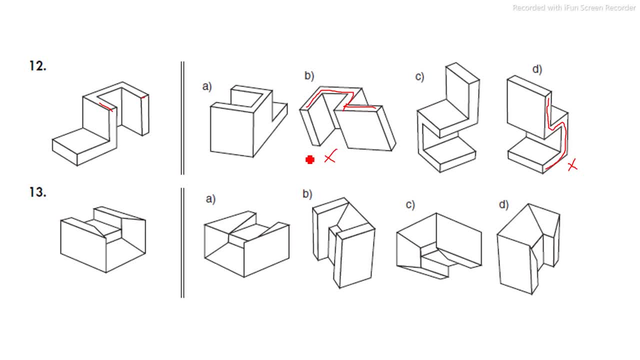 things. so we'll have to figure it out whether they are mirrored or not. so we'll have to figure it out, structure or not. so if you see here this is, if you try to un think like you are standing in this gap, we were standing in this gap and you are facing this wall. you are seeing, this is green. 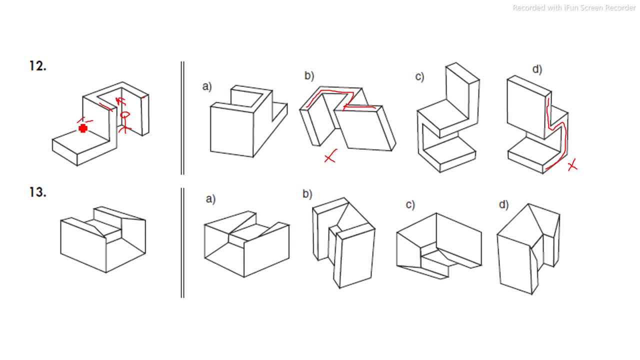 so this L like structure will come to your left hand side and similar thing. if you try to do with this like if you think you are standing here, so you just can't your head and try to imagine that you are standing here and you are seeing this wall. so this l like 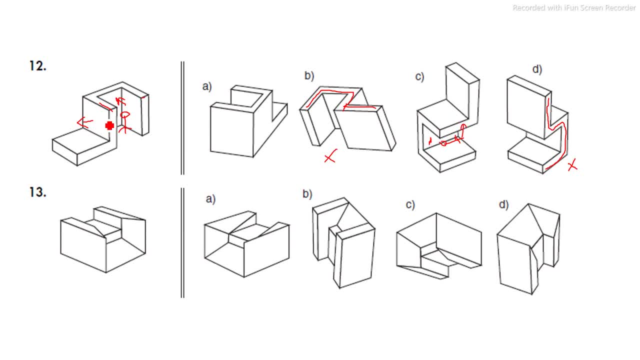 structure will come to right hand side, right, and here it is coming to left. so this is a mirror image, so this will be eliminated, so this will be our right answer. coming to question number 13, so here you can see this, uh, this, uh something. a pointed structure is like there, right, this pointed like 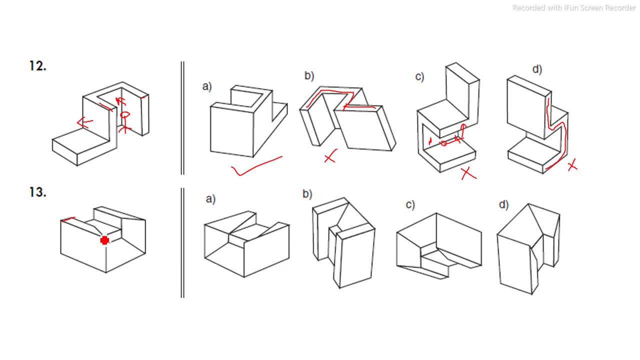 structure will try to figure out whether we can eliminate based on this or not. so this is completely ruled out. because you can. you cannot see this kind of pointing structure. this is ruled out here. if you see, this is not at all pointing at all. this is a complete rectangle structure. so 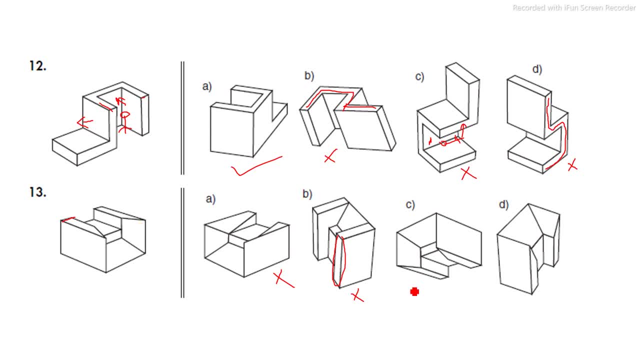 this is eliminated. here you see, these similar structures are there. so this can be our answer here. also the similar structure there. this can be our answer now. moving on to the second point, if you see here there is two line structure, a solid structure, is there something which is having a borderline of two? 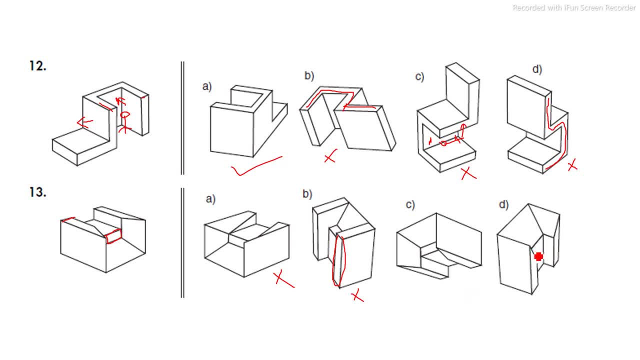 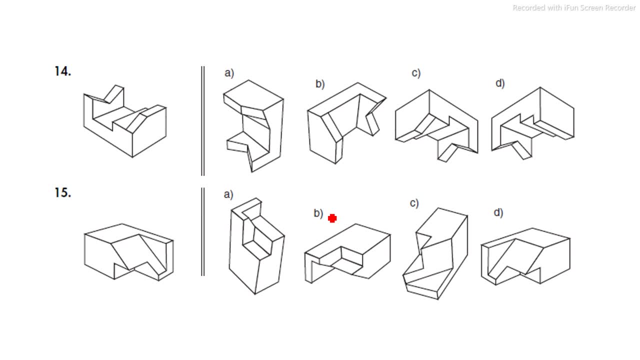 layers and here, in this figure, only one layer is there. one layer is missing. so this is eliminated. so this is our answer. coming to our next slide, in this figure you'll try to rule out by elimination method. so what we see here is that this is, uh, this, this kind of thing, and this is so based on this. 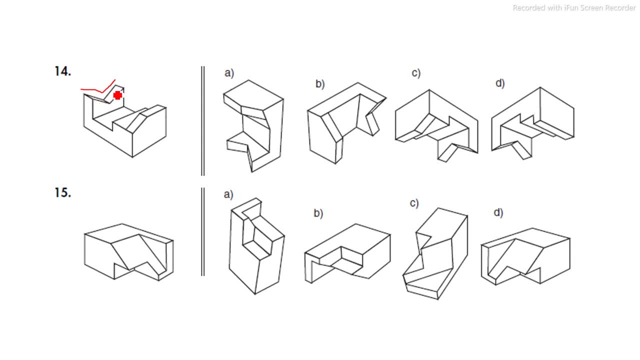 structure. there is some kind of double line and there is a rectangle. so you'll see a double line and a rectangle double liner, rectangle double line and rectangle double end. so it is all of there. now i will go with this. a slope is there here. a slope is there here also. slope is there. 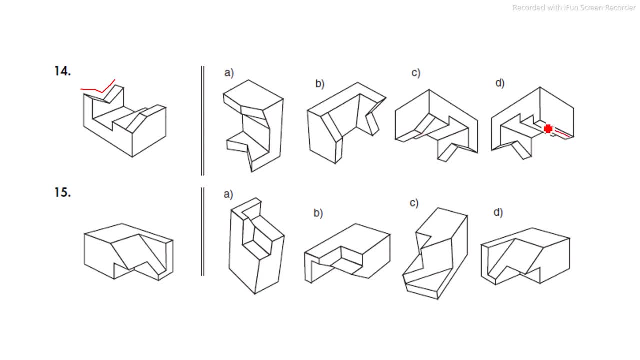 here also slope is there, but here we see a complete rectangle. so one elimination we found. now we go on to next thing. so what can be our next thing? so? so if you go by this structure, you'll see this one. we'll try to find out whether these are there in this picture or not. you can see with this this: 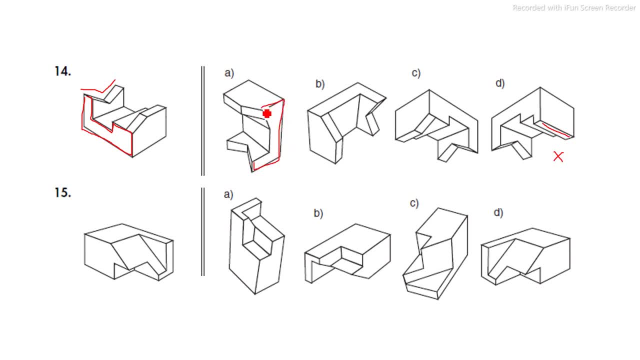 structure is not there. this structure is completely different. like here: if you're sloping, here we are having a downward step arrow, but here, if you see, this is inclined one. so this is eliminated. here, if you see, this is going good, but here this complete wall is missing. here, right. so here till now it is good, but this: 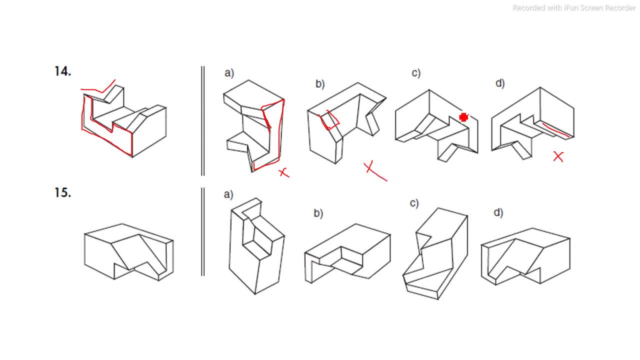 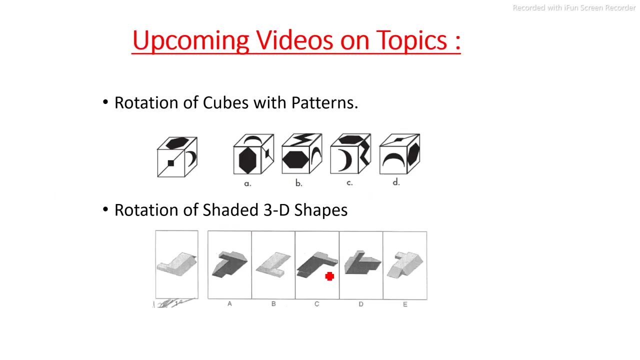 complete wall is missing. so this is not our answer. now, here we can see this, this is a. this can be our answer, right, and here also, if you see, but in, oh, this is all always. this is already eliminated, this eliminated, this eliminated. so this is our answer. learn about the rotation of hues based on patterns, this kind of 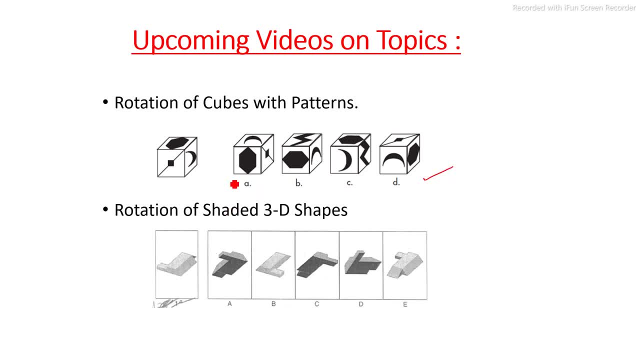 figures and then in next to next video we'll learn about rotation of shaded 3d steps. so these are a bit quite analytical. you'll have to analyze things a bit because these are the shaded regions. you'll have to focus where the shaded regions are there and which one are the lighter regions. so we'll see. 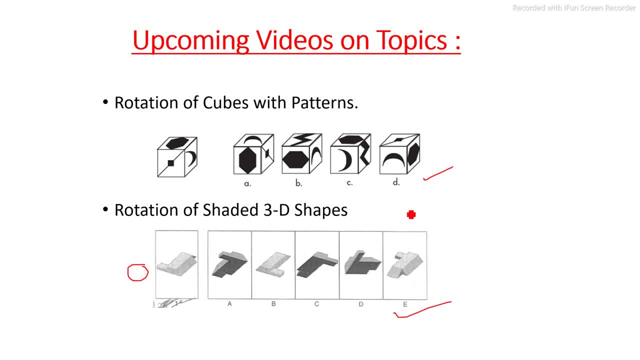 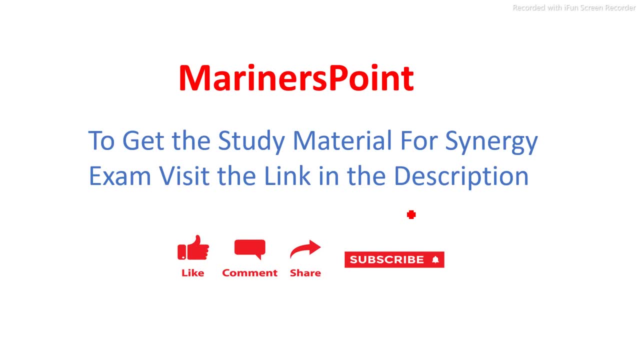 what we can do in this kind of things. and so for this, and if you like this video, please share it with your friends so that you can also understand that these concepts clearly. and please do comment if you want to make us video on any other topic, if you are facing any difficulty on any other topic also, you